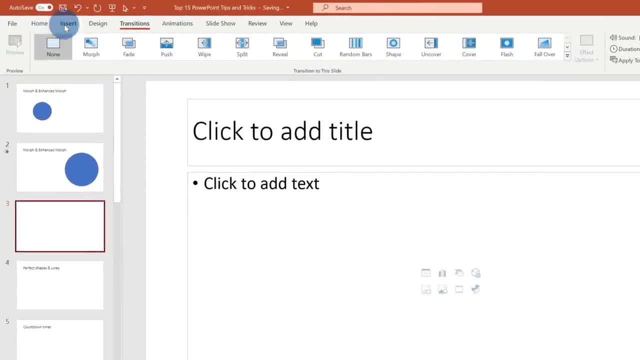 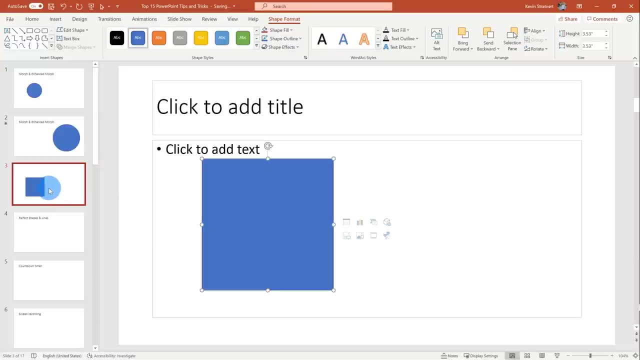 I'm going to insert another slide and on this slide I'm going to go up to insert on the ribbon. Here I'm going to click on shapes and I'm going to insert a rectangle. Now I want this circle to morph into this rectangle. How do we do this? Well, first off, on slide three, let's click on the slide. 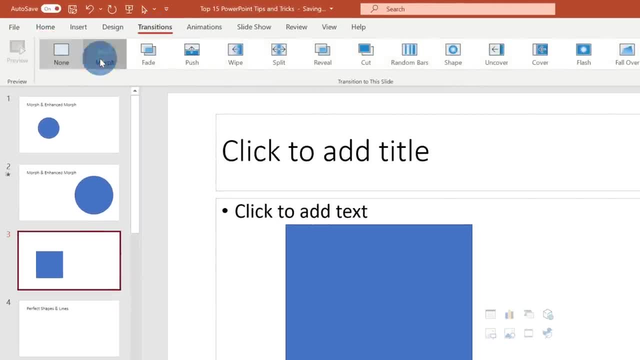 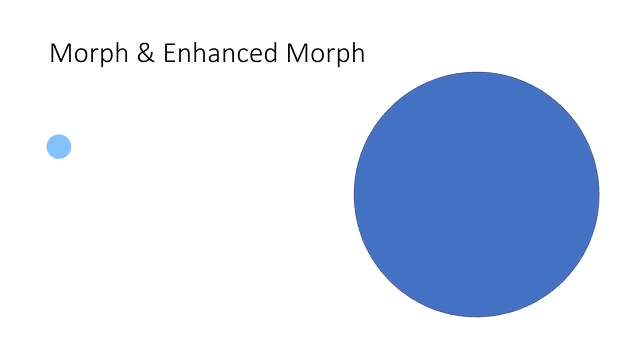 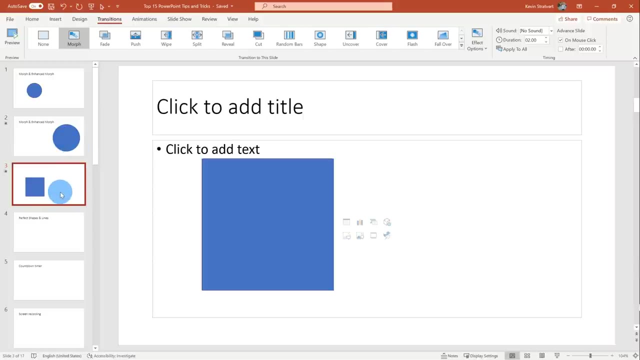 and then go up to transitions. Once again, I'm going to click on morph, but right now we see that I'm in the selection mode. There I get my bigger circle and there it simply fades in and out to the rectangle. How do we get the circle to morph into a rectangle? Well, we need to ensure that both the 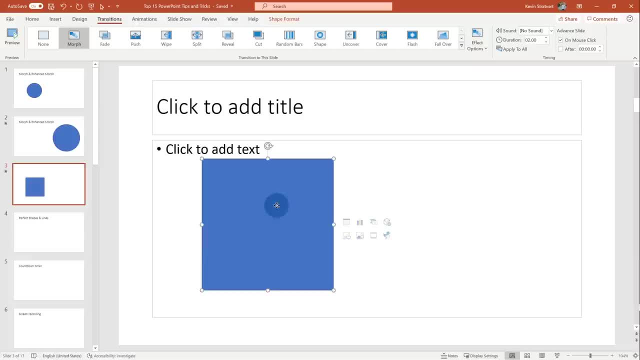 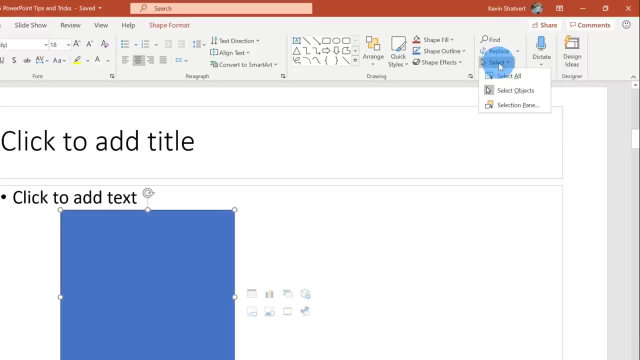 rectangle and the circle share the same name. To make sure that they share the same name, let's click on the rectangle, then click on home on the ribbon, and we're going to go over to the selection pane. I'm going to click on select and then click on selection pane Within the selection. 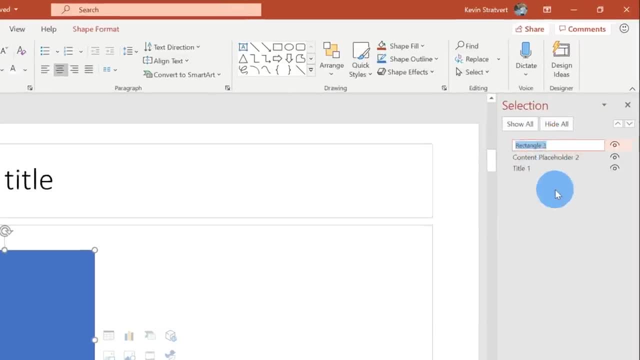 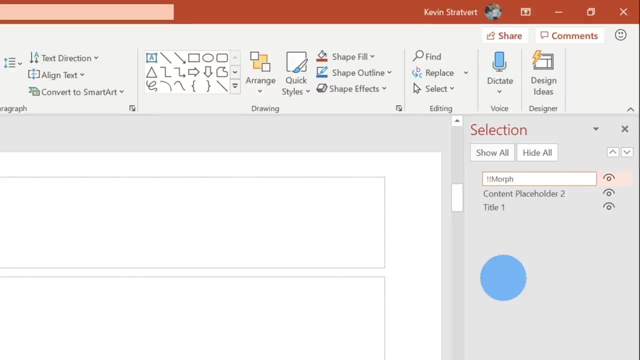 pane. I see that my rectangle simply has a name: rectangle three. I'm going to change this name and we need to insert exclamation marks. I'm going to insert two exclamation marks and then I'm going to type in morph To do an enhanced morph. you need to make sure that you include. 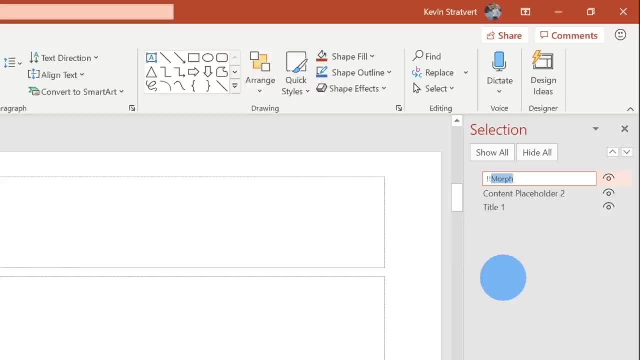 exclamation marks, but the name itself doesn't necessarily matter. You just have to make sure that this name matches for the shape here and the shape that you want to morph from. I'm going to copy this name, and now I'm going to jump into slide two. I'm going to click on the circle here. 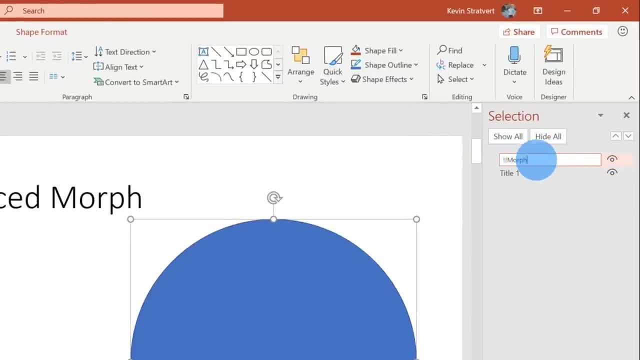 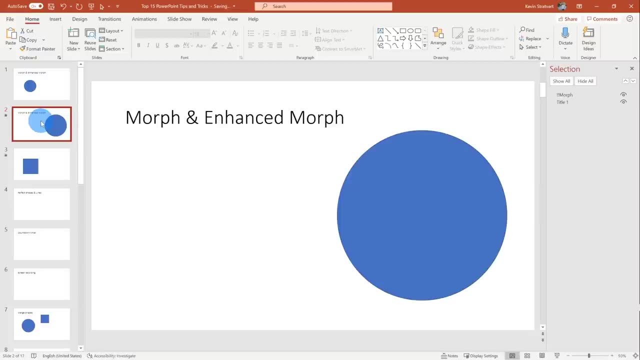 and with the selection pane open, I'm going to click in here and paste in the same exact name. PowerPoint now knows that it should morph this shape into the rectangle. Let's jump in the presentation mode again and see how this looks. I'm now on slide two, and let's jump into slide. 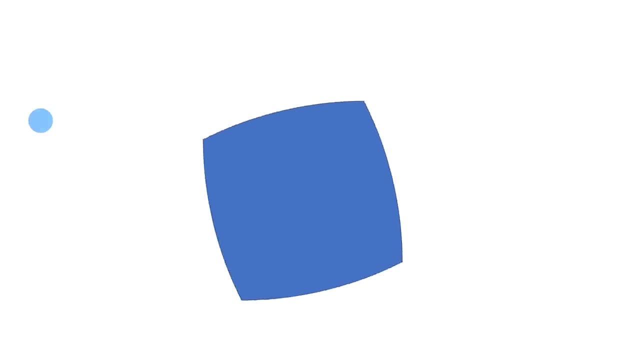 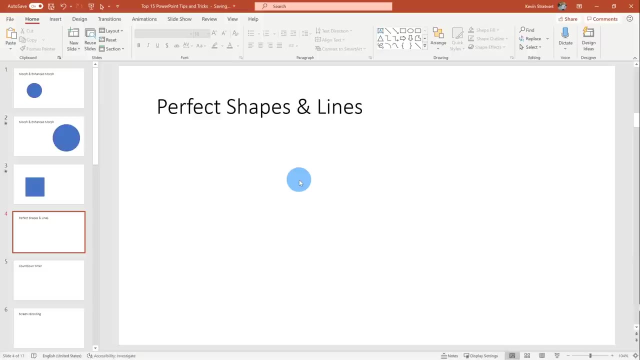 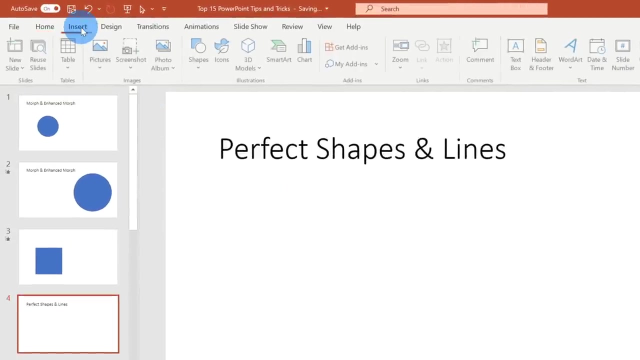 three. There you see the circle morph into a square. That is a pretty cool transition, and that's tip number one. Tip number two: I want to show you how you could insert a perfectly symmetrical shape and also lines. To do this, first off, let's go up to the ribbon and click on. 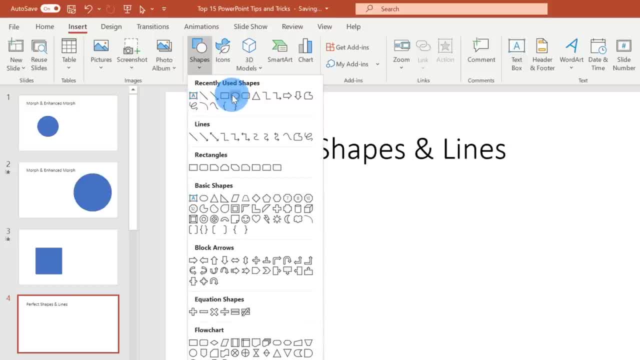 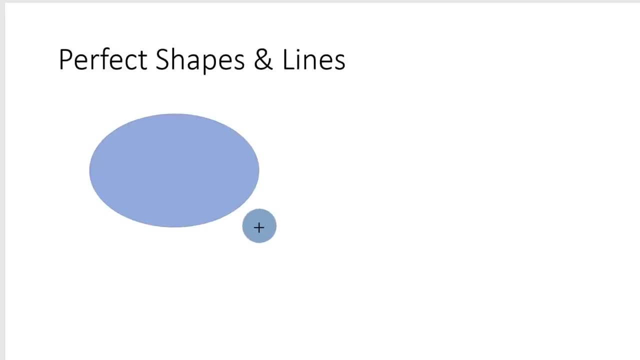 insert and then click on insert. I'm going to click on insert and then click on insert. Then we're going to click on shapes. First I want to insert a circle or an oval. I'm going to click on this and here I'm going to start drawing it on my slide. Now, if I want to make 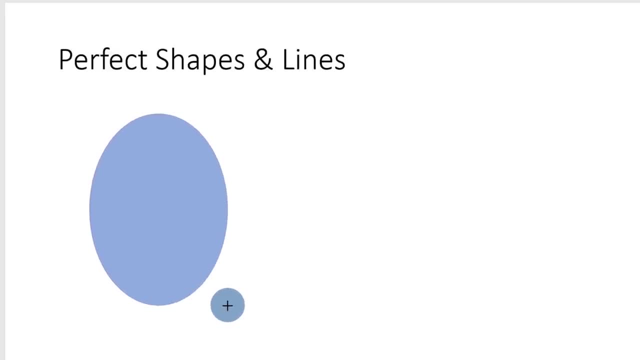 sure that this is a perfect circle. I could try to line it up, but I might not be quite right. If I want to ensure that I have a perfectly symmetrical shape, I can simply press the shift key and this will ensure that I have a perfect circle. I could use this for any type of shape. 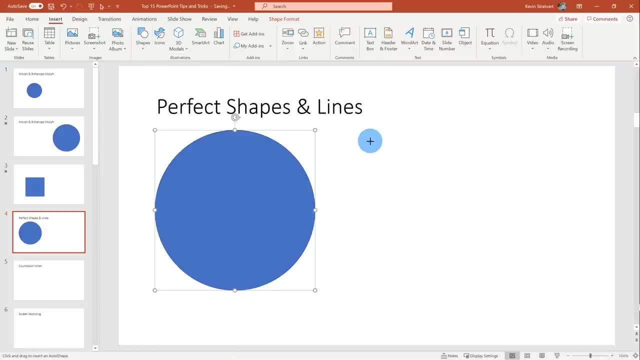 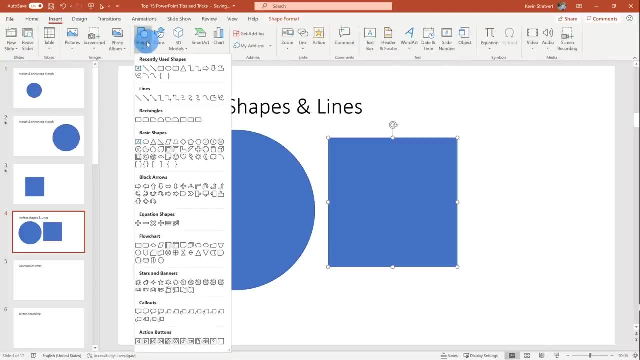 I'm going to go back to shapes, and now I'm going to insert a rectangle. I'll press the shift key and here now I have a perfect square. Now not only can I use it with circles or squares, I could also click on shapes and I could use it for lines. Here I'm going to insert an arrow. 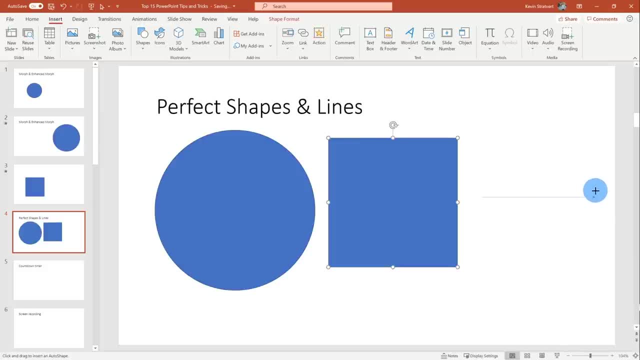 and I'm going to press the shift key again, and this ensures that I have a perfectly straight line. If I didn't use shift, it'd be a little hard to align it. Now, if I press shift and I go up, it'll move in 45 degree increments and give me a line. So here, this way, 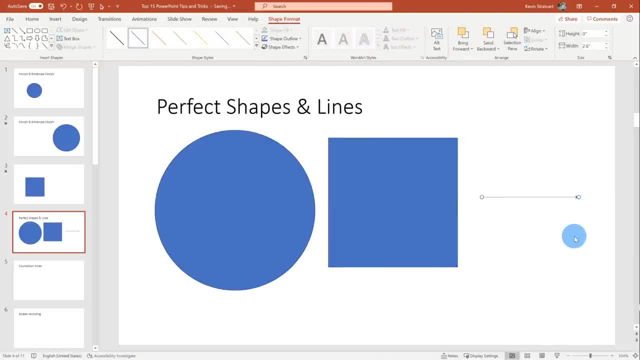 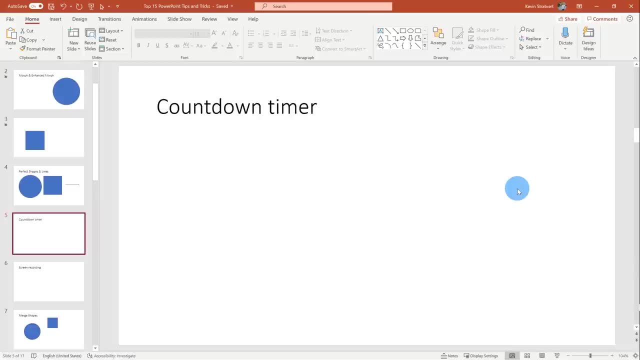 I could get nice clean lines on my slide. This is tip number two. Tip number three: I want to show you how you could insert a countdown timer into your PowerPoint presentation. Oftentimes you're presenting in front of a group and maybe you 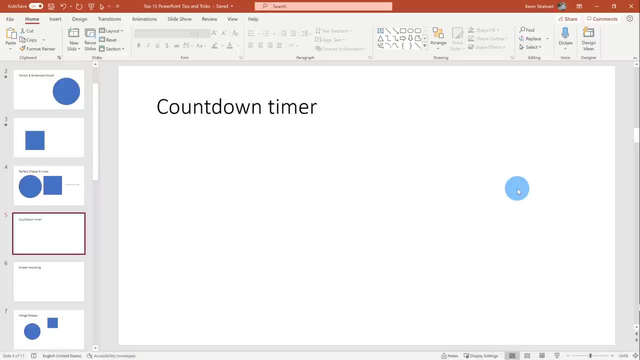 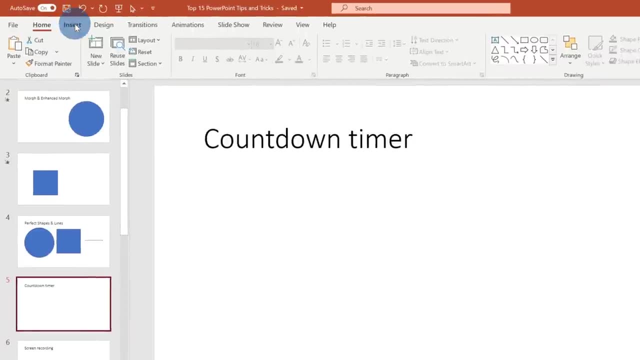 want to take a short break and you want to let your audience know how much time they have. Luckily, it's very easy to insert a countdown timer into PowerPoint. Within PowerPoint, go up to the ribbon and click on insert, and then we're going to go over to the add-in section. 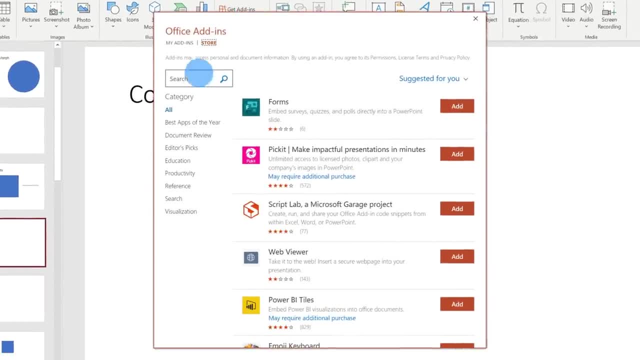 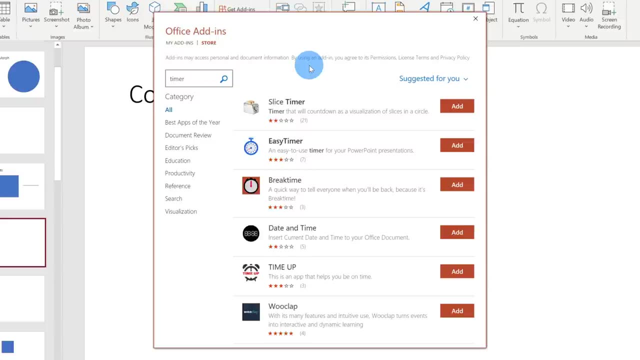 and we're going to click on get add-ins Within the office add-ins prompt. let's click on search and we're going to type in timer and then search. This shows you a number of different timers that you can insert into your PowerPoint presentation. I personally like the break time. 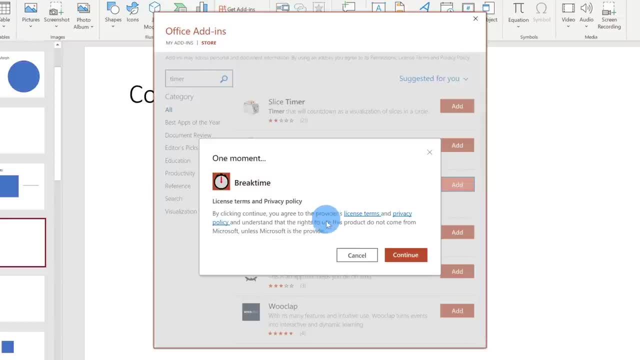 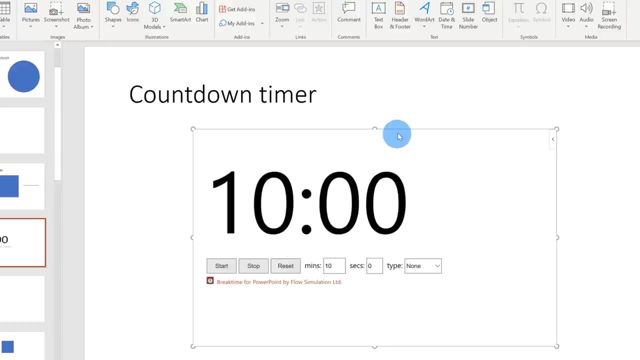 timer. I'm going to click on add for that. Next, it'll ask me to agree to the license terms and privacy policy. I'm going to click on continue Next. this inserts a countdown timer into my slide. I could position it however I want it to appear. I could set how much time I want the 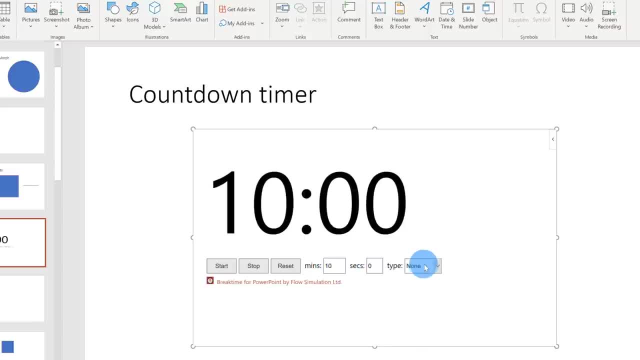 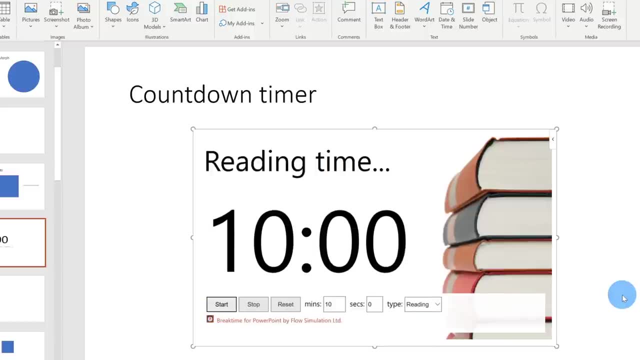 countdown timer to be for Here. by default, it's set to 10 minutes and zero seconds and I could choose a background that I want to apply. I'm going to select reading, Next I'm going to click on start and we could see what the breakdown timer looks like. This is a cool, neat little. 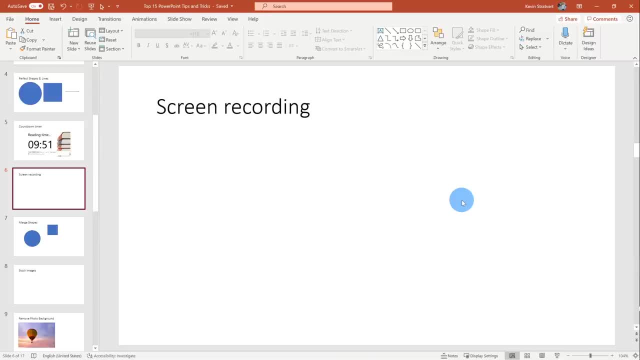 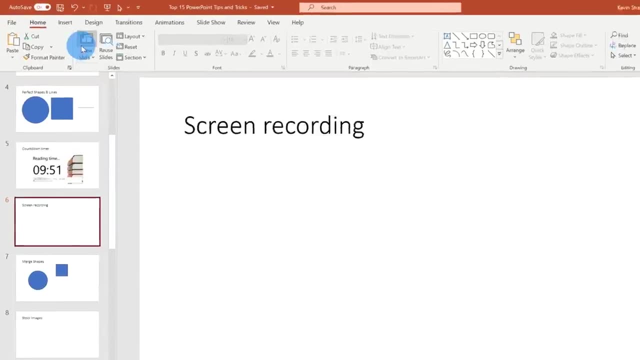 tool that you could implement into your slide to have a timer. Tip number four: you can record your desktop or your screen using Microsoft PowerPoint. To record your screen, go up to the top ribbon, click on insert and all the way over on the right-hand side you'll see an option for screen. 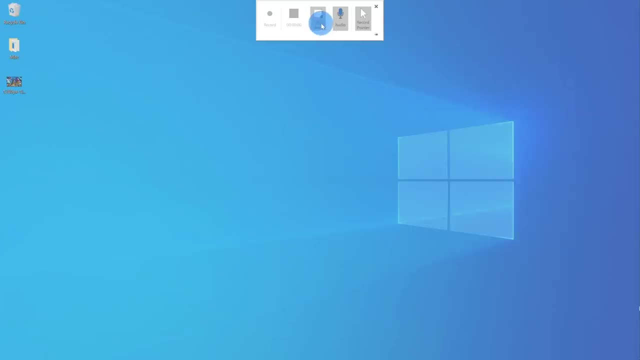 recording. If we click on this, this will drop me on the desktop. I could select the area of my desktop that I want to record. I'm simply going to select the entire screen and then I'm going to click on record. It shows me the shortcut key that I could press. 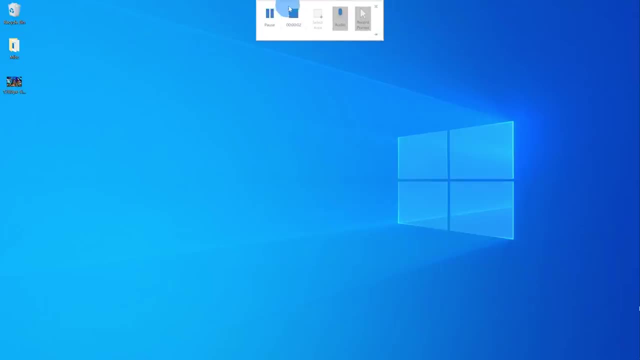 Windows logo, shift and Q to stop the recording, or I could hover up above to stop the recording this way as well. Now I could click on an item on my desktop. Here's a nice picture of Times Square, and now I'm going to press Windows logo, shift and Q and that'll stop the recording. 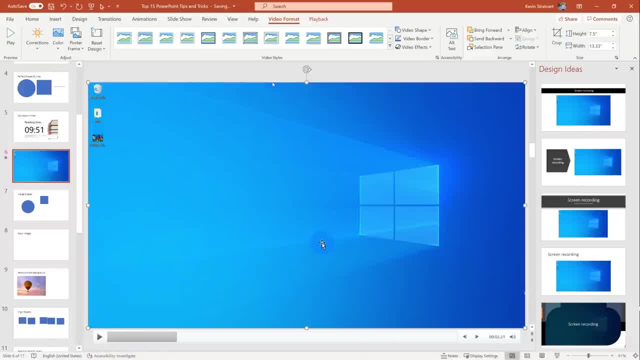 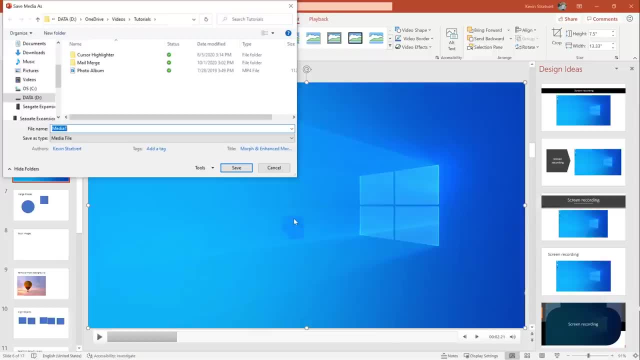 You now see that my screen recording is inserted into Microsoft PowerPoint. Now, I'm not just going to use this screen recording in PowerPoint, I could right-click on it and I could also save this screen recording as an mp4 if I want to use this elsewhere. So pretty awesome functionality. 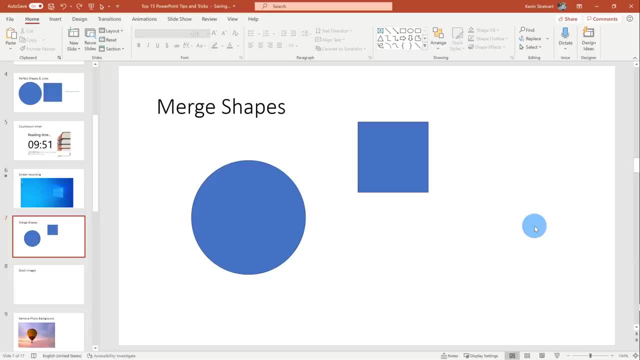 built directly into PowerPoint. Next, I want to show you how you can merge shapes On this slide. I have two different shapes. I have both a circle and a square. I'm going to pull my square and I'm going to position this over my circle and I'm going to put it right about there. 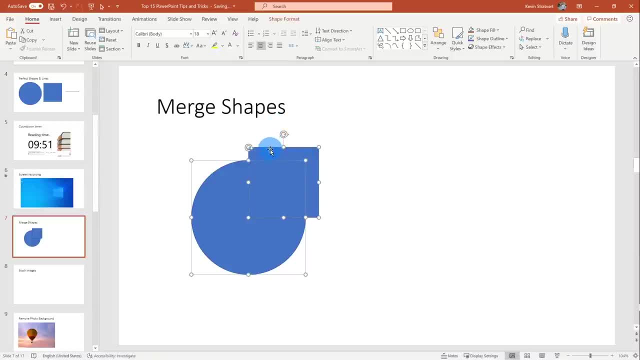 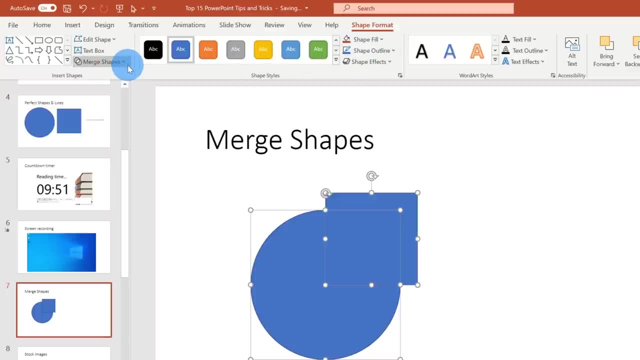 Next, I'm going to select both of these shapes and because I have shapes selected, I see the shape format option on my ribbon. Let's click into that Now over on the left-hand side. because I have multiple shapes selected, I have the option to merge shapes. 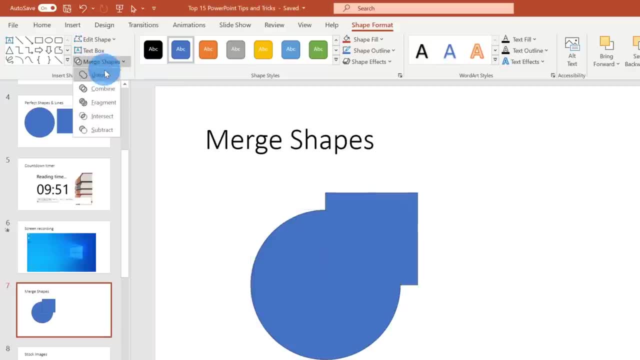 When I click on this, there are many different ways that I can merge these shapes. For instance, I can do a union, where I bring them together into one shape. I could also do a combine, where it leaves out the intersecting portion of it. I could also do a fragment, where it creates three separate. 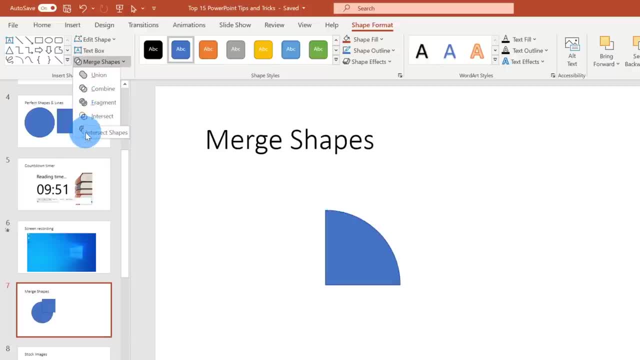 shapes. Here. I could do an intersect where it just keeps the intersecting portion and the last to subtract the second shape from the first one. I'm going to go with fragment to see how this works. Now that I've done fragment, I have three different shapes. I'm going to remove this portion. 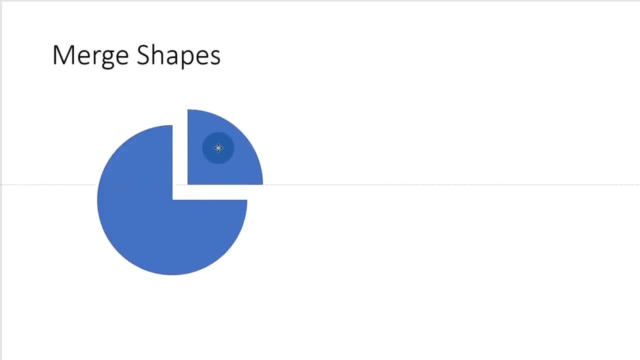 for now and I'm going to delete that. Next, I'm going to pull out this portion of my circle. This could be a neat technique. Say, for example, in a presentation that I have this pie that maybe represents all of our sales. and I want to have a point out at this portion of the circle calling 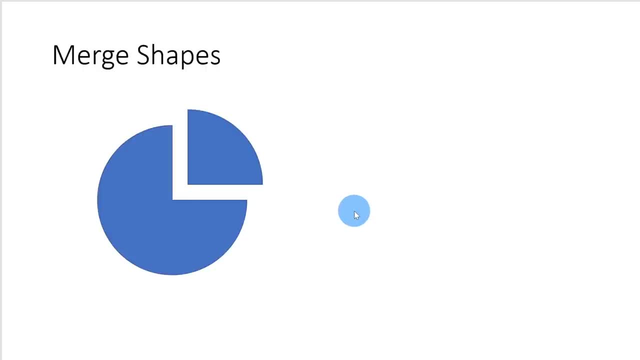 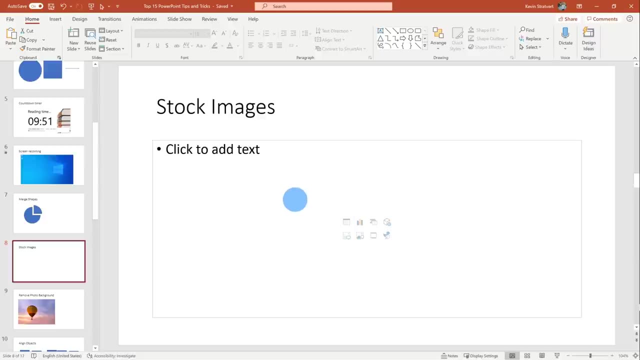 out what happened with this portion of our sales. You could do lots of neat things with merging shapes. Tip number six: Microsoft PowerPoint has a whole bunch of different stock images that you can insert into your presentation. To insert stock images, simply go up to the top ribbon. 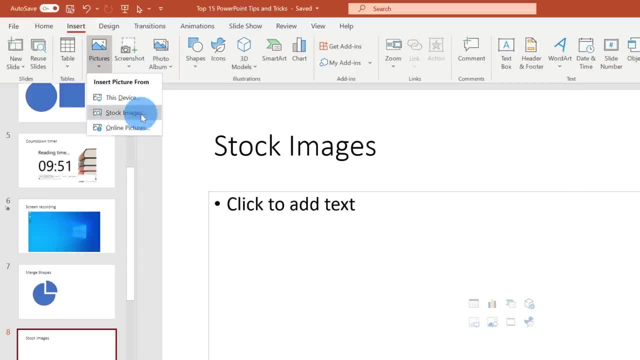 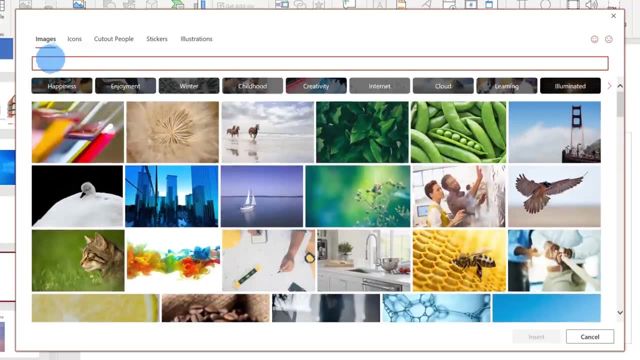 click on insert and then click on pictures, and then within pictures, there's an option for stock images. When you click on this, you have a massive variety of stock images that you can bring into your presentation. You could search for images, you could click on categories or you could simply. 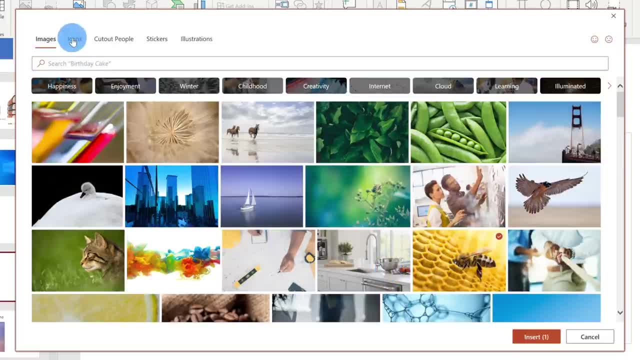 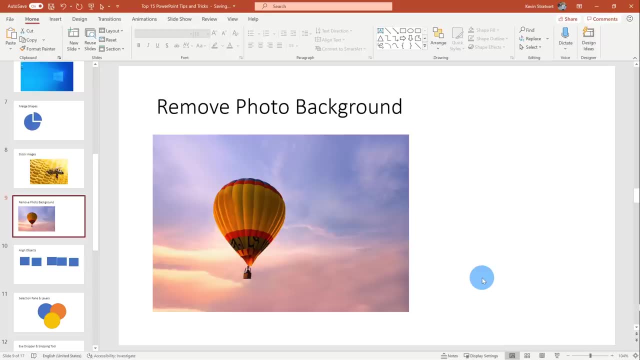 click on an individual image. Along with clicking on an image, you can also insert icons, cutout people, stickers and illustrations. I'm satisfied with my selection. I'll go ahead and insert this Here. you see, a very high resolution photo is inserted onto my slide. 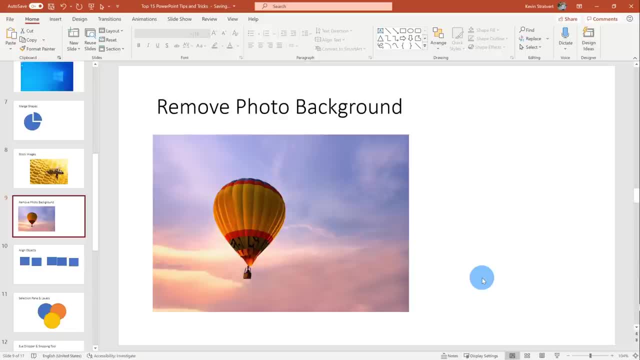 Tip number seven: did you know that you can remove the background from a photo? Here I have a beautiful picture of a hot air balloon and I want to remove the background sky. I'm going to select the photo and I have the picture format option on the ribbon When I click on that over on the left. 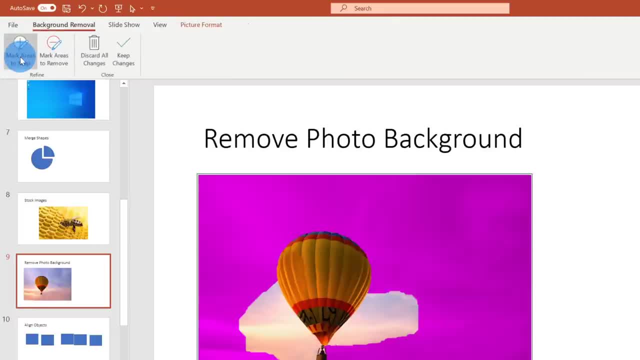 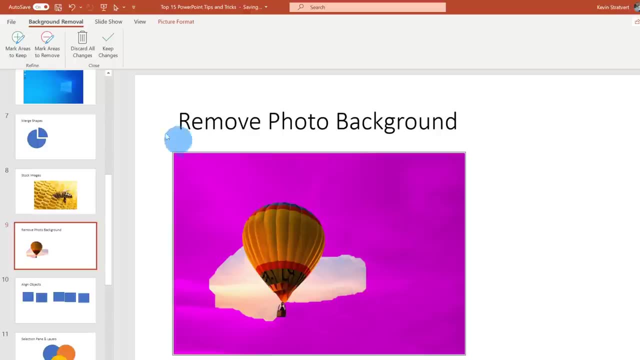 side I have the option to remove the background. I'm going to click on that. This now does its best job at removing all of the background, but I see that it hasn't quite removed everything. If I go up to the ribbon, I could click on mark areas to remove and then I could highlight the section of 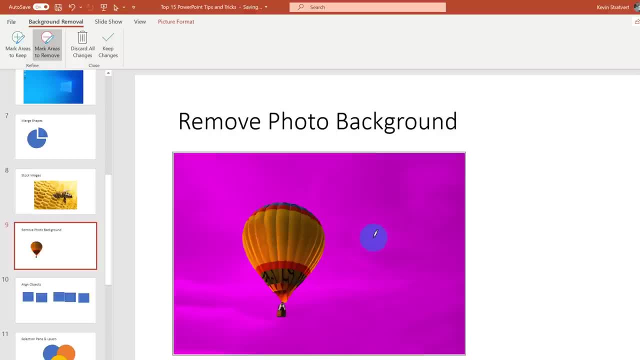 the image that I want it to remove Here. I'll click over here, and that removes that background as well. Now you can see there's a little bit of background left behind the bucket of the hot air balloon, so I'm just going to click in there to remove that as well Once I'm satisfied with the. 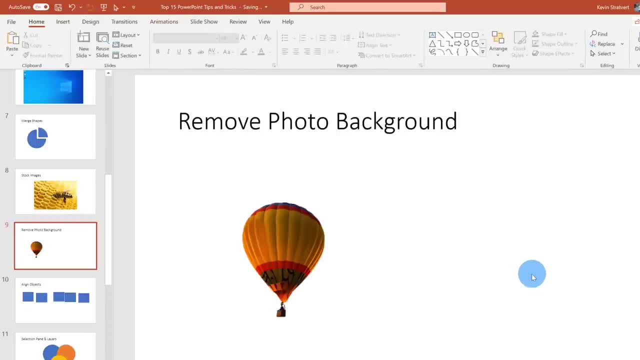 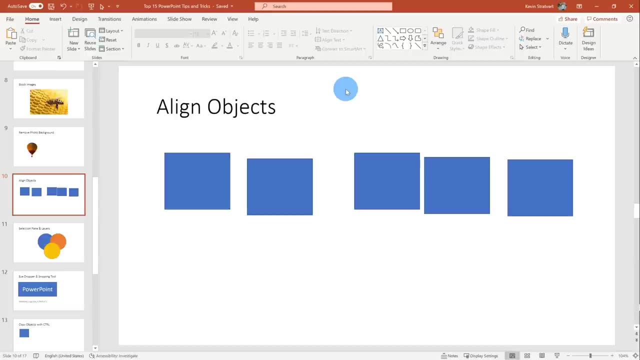 all of the results, I can click on keep changes. and that's now removed the background from my hot air balloon. Tip number eight: I want to show how you can align objects on your slide like a pro. To align these objects, first off, let's highlight all of these squares. Once we have them highlighted, 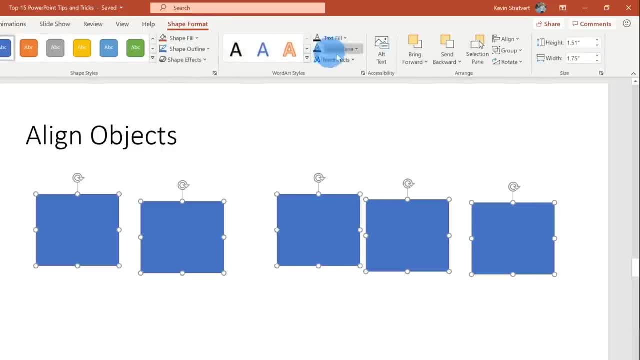 let's go up to the top ribbon and click on shape format. Over on the right hand side we have the option to align. I'm going to click on align and first off, I want to top align all of these shapes. Click on that first. Now I see all of the items are top aligned. I'm going to click on align again. 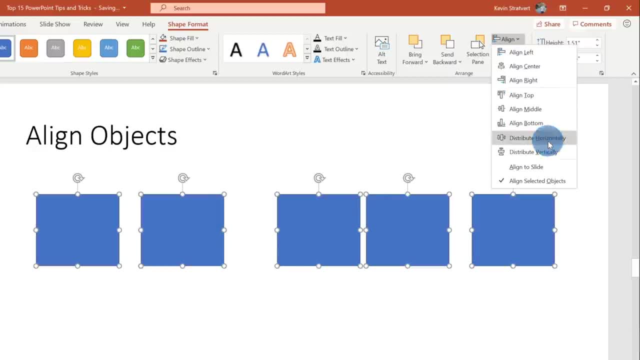 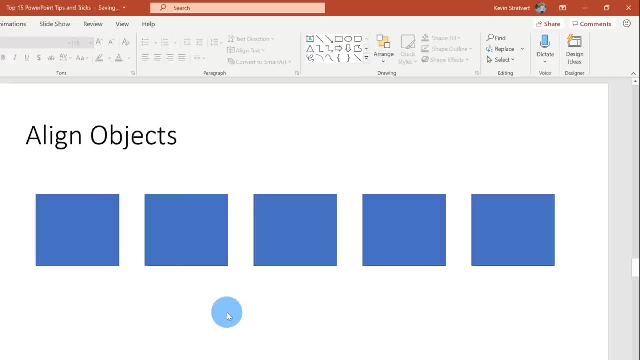 and I want to distribute horizontally to remove these big gaps between the items Here. now you can see that they're all top aligned and the spacing between each item is identical. This now looks very nice and I was able to effectively align my objects. 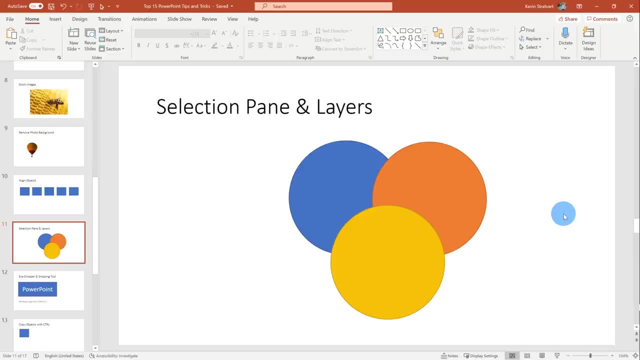 Tip number nine, I want to show you how you could use the selection pane and work more effectively with layers. You see that I have three different circles on my slide. I have a blue circle at the bottom layer, then a red circle in the middle layer. 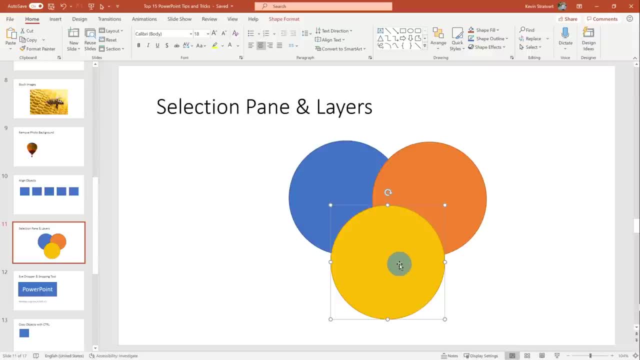 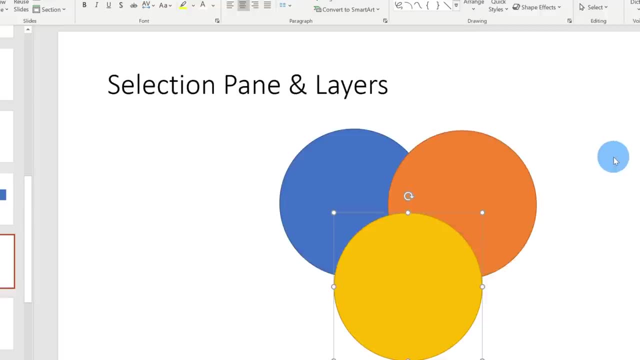 and my yellow circle is on the top layer. To move these different items between layers, you could simply right click on them and you could send it all the way to the back, or you could simply send it one layer back. Now, this could take time, especially if you 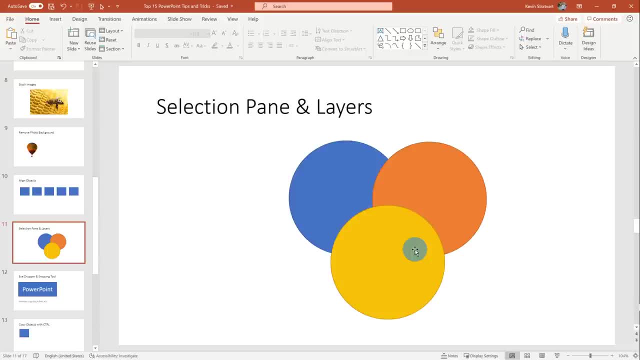 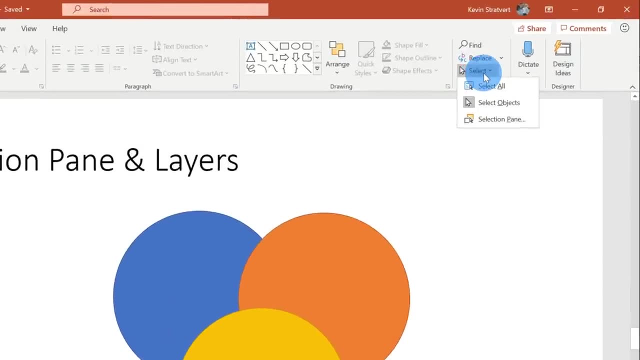 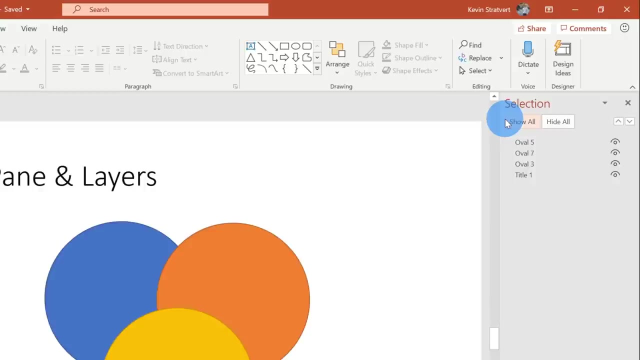 want to modify lots of different items on lots of different layers. To work with this more effectively, let's go to the home tab on the ribbon and then, over on the right hand side, click on select. Within the selection menu there's an option called selection pane. Let's click on that. This opens up the selection pane. 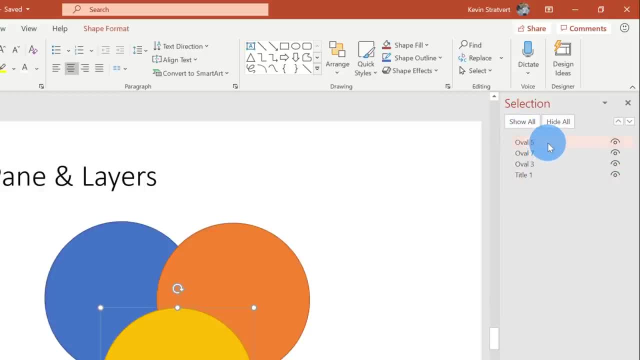 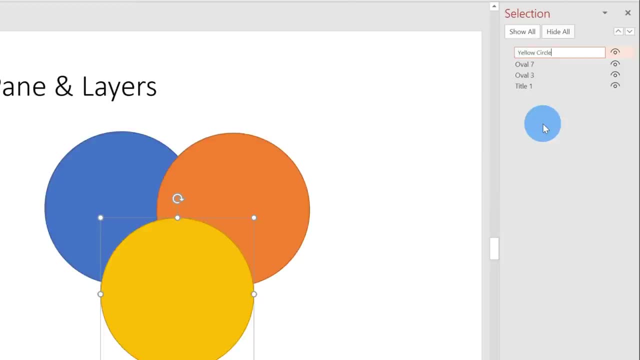 and I see all of the different objects that I have on this slide. For instance, if I click on oval five, it turns out that's the yellow circle. If I double click, I could rename this object. I could go through now and I could rename all the objects on this slide to make it easier. 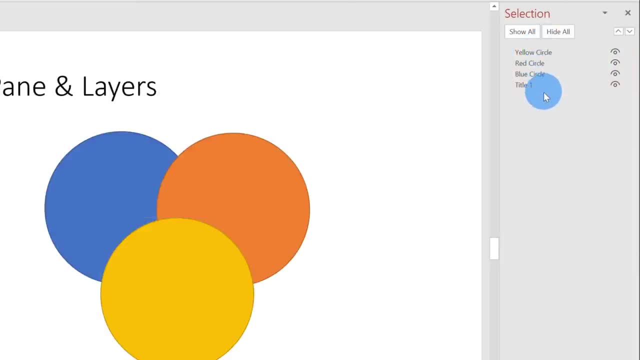 to know which item is on which layer. I've now renamed all of the different objects within the selection pane, so now I very quickly and easily know which object is which item. here I could hide items within here. Let's say I want to hide the yellow circle. 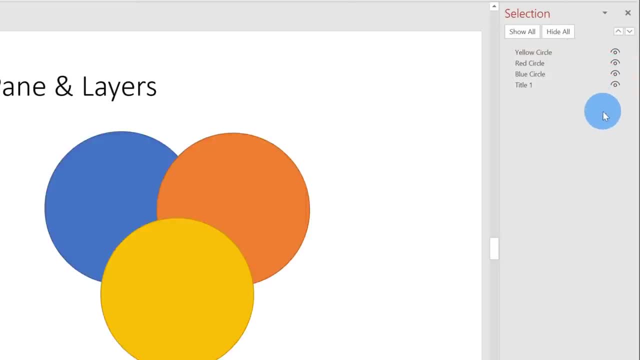 so maybe I could work on the red circle and the blue circle and then I could show the yellow circle again Now to move items between layers. whatever item appears at the top of the list is on the top most layer. I could click on this item and I could bring the yellow circle to the 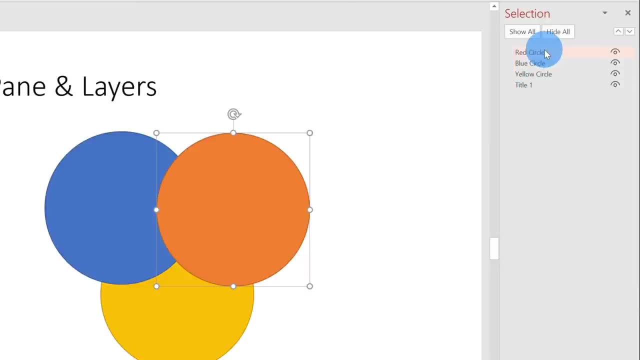 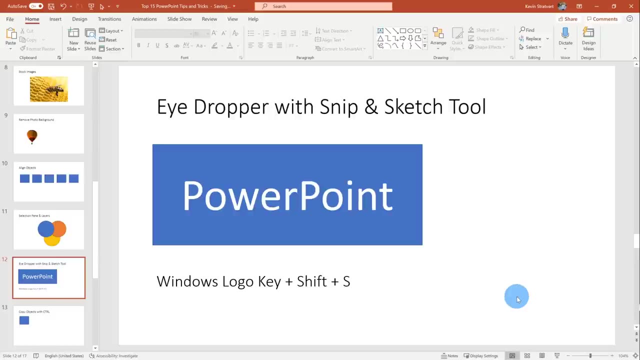 bottom, or maybe I want to move the red circle down. I could very easily do that by dragging and dropping items within the selection pane. Tip number 10,. I want to show you how you can use the eyedropper together with snip and sketch. 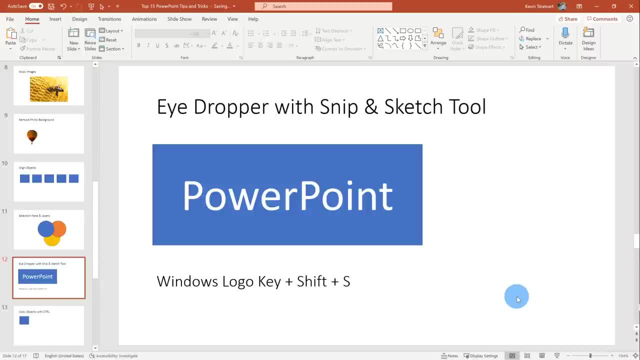 To be able to copy any color that appears on your desktop. I have a rectangle in the middle of my slide and it says PowerPoint, but this isn't the PowerPoint brand color. I see the brand color up here on the top app bar. 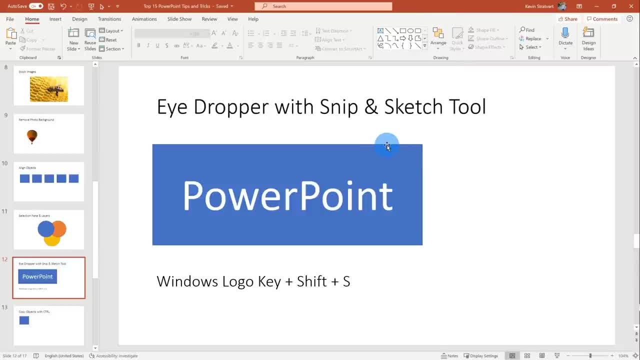 How do I get this color into the rectangle? Well, first we're going to use the snip and sketch tool. This comes with Windows 10.. To launch snip and sketch, we're going to press the Windows logo key together with shift and S at the same time. This launches the snip and 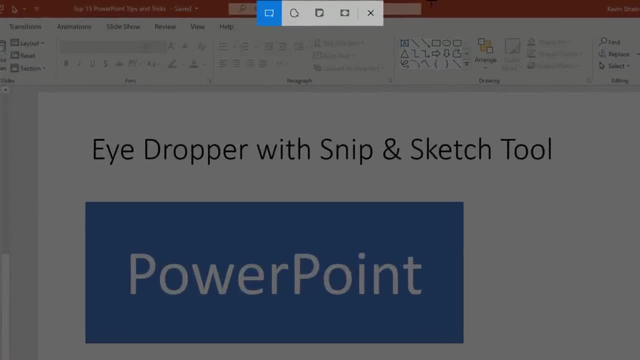 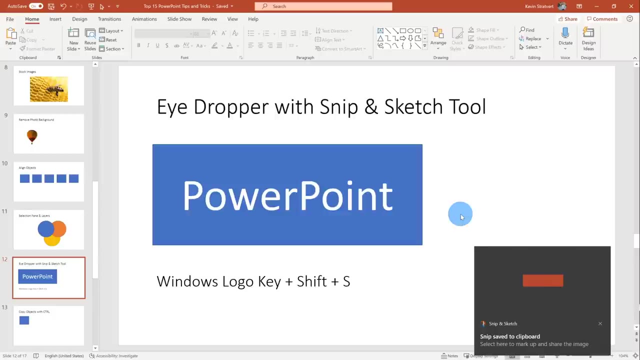 sketch tool and I'm going to go up here and select a rectangular snip. Now I'm going to draw a rectangle around the top app color. I see now that this color is on my clipboard. Next I'm going to click into PowerPoint and I'm going to press control V. 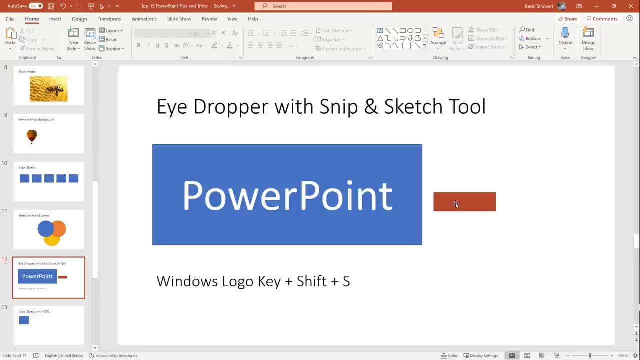 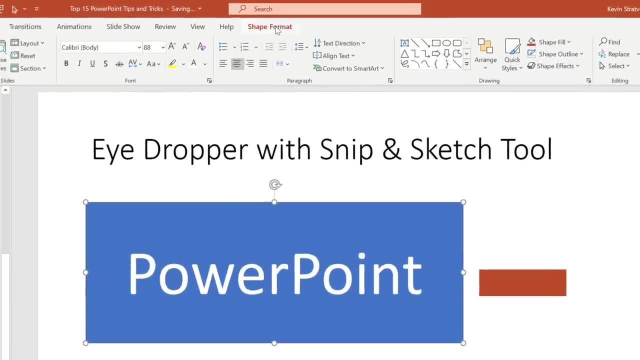 to paste this onto my slide. This pastes the app color onto my slide. Next, I want to take this color and get it into my rectangle. I'm going to click on the rectangle and go to the top bar to shape format. Within shape format, I'm going to click on shape fill, go down to the 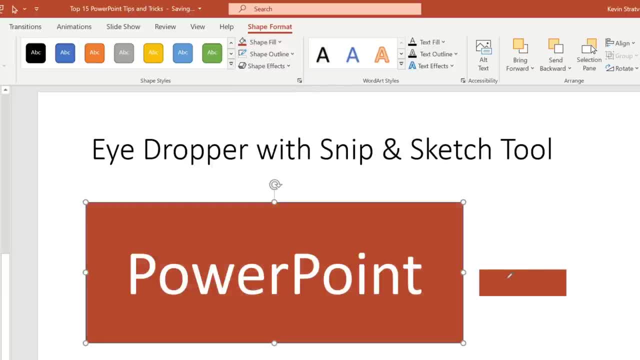 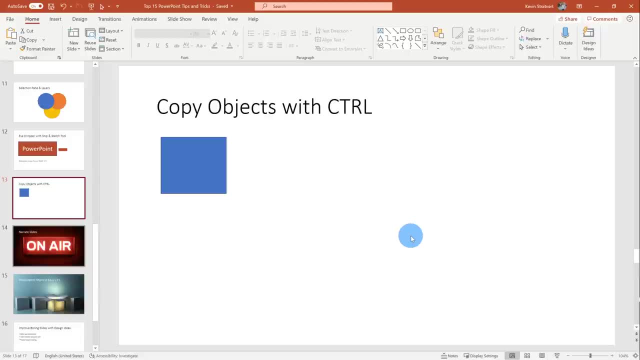 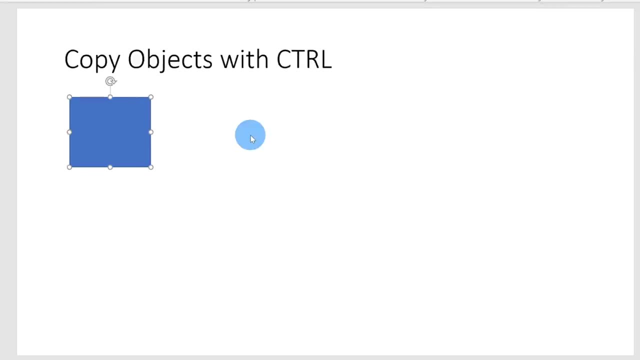 drop or tool and I'm going to select the color from this rectangle. This now applies the same exact color from the top bar to this rectangle. Tip number 11, I want to show you how you can copy objects using the control key. I have a rectangle on the slide and I currently have it selected. 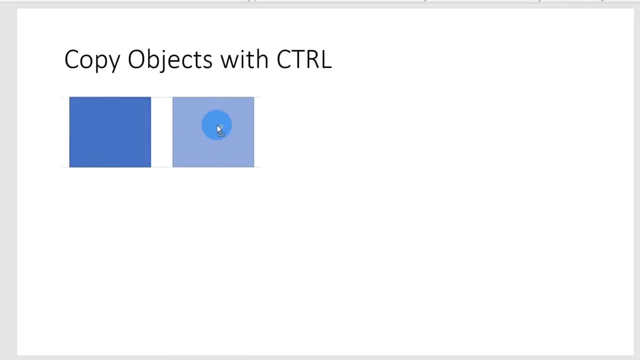 If I press the control key and then click on the object and drag it over, this will give me a copy of the object. I could also select multiple items, So here I could highlight both items and I could press control and then drag down and that'll give me two copies of the item. I could also 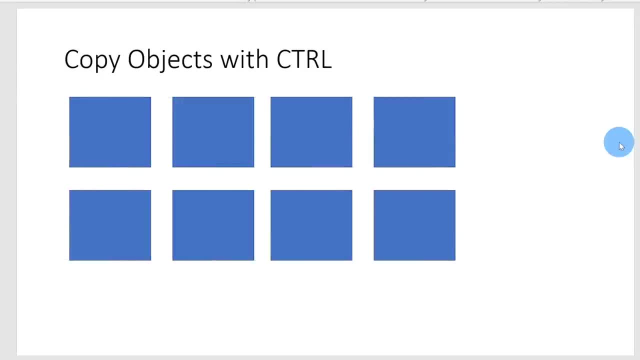 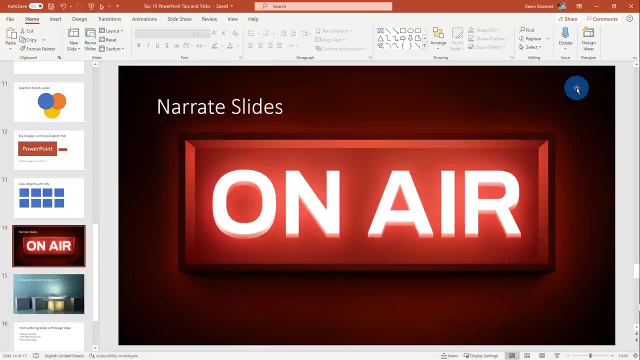 select all four of these press control, and now I have a whole bunch of copies of the original rectangle. Tip number 12, did you know that you can narrate PowerPoint slides together with your voice and also video? To narrate a slide, let's go up to slideshow on the top ribbon and then 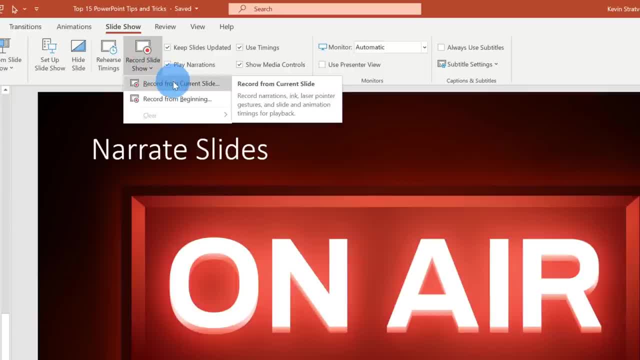 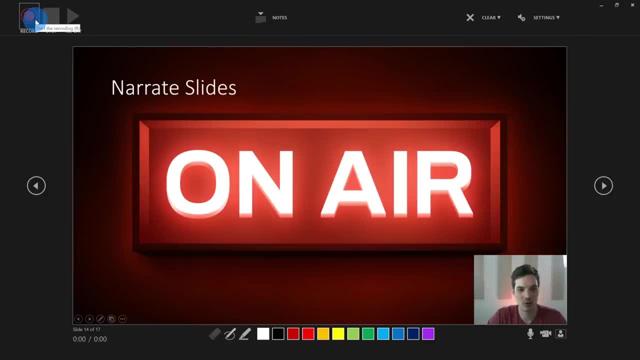 there's an option to record a slideshow. We could record from the current slide or from the beginning. I'm going to click on record from current slide. It opens up the record interface. I could click on record, I could also go through and I could. 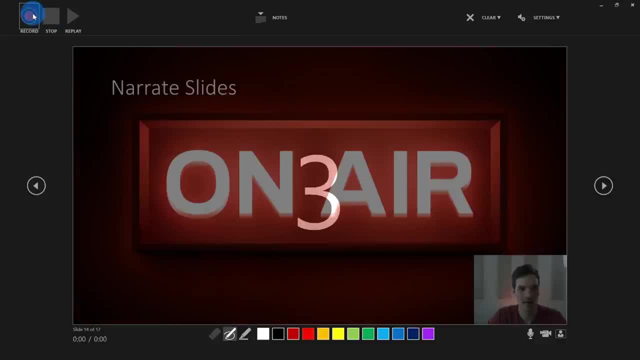 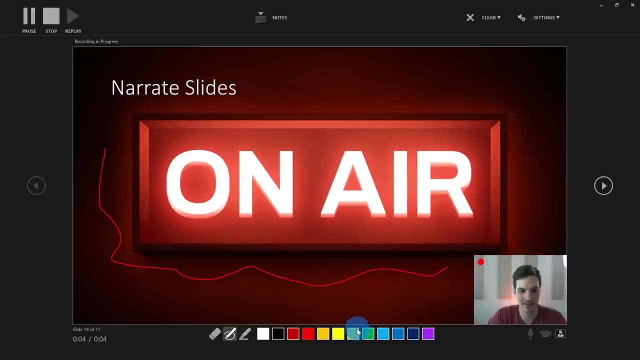 annotate my screen. Let's click on record to see how this works. I'm going to click on record. I see a countdown message and hey, we are on the air Here. I'm going to annotate the slide. Maybe I'll insert a different color and this sounds great. Once I'm all done, I'm going to click on the stop. 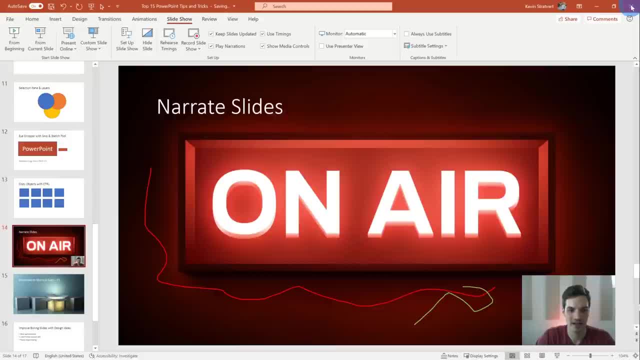 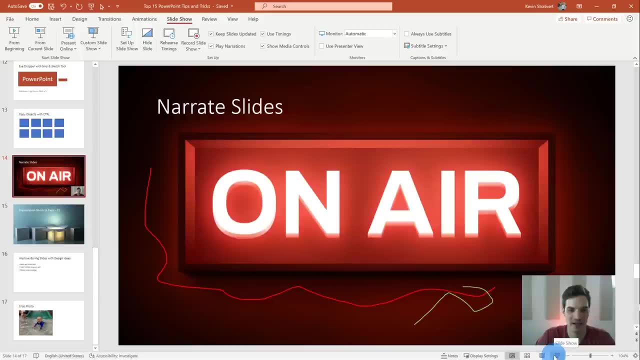 button on top. Next I'm going to click on the X in the top right-hand corner, and now this inserts my video and my annotation on the slide, Tip number 13,. if I jump into presentation mode, you'll see the slide come up with my annotations and the video will play. 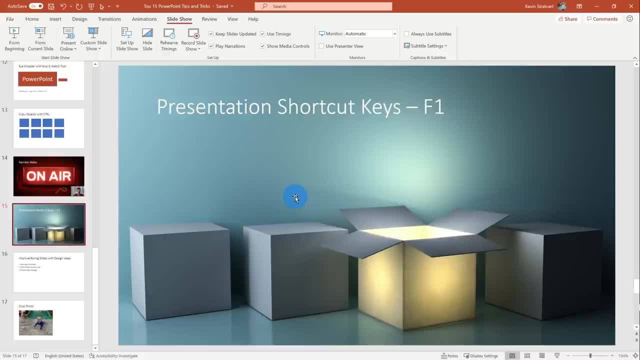 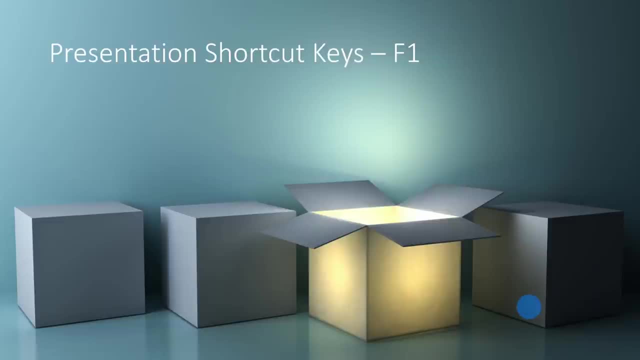 Number 13,. when you're presenting in Microsoft PowerPoint, there are all sorts of shortcut keys that you could use in presentation mode. First off, let's jump into presentation mode. If you press the F1 key, this will show you all of the different shortcuts that you can use when you're 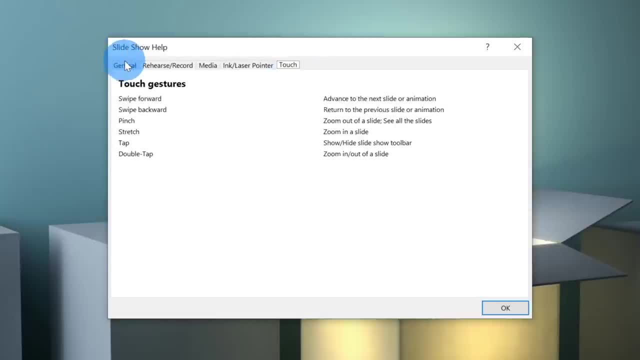 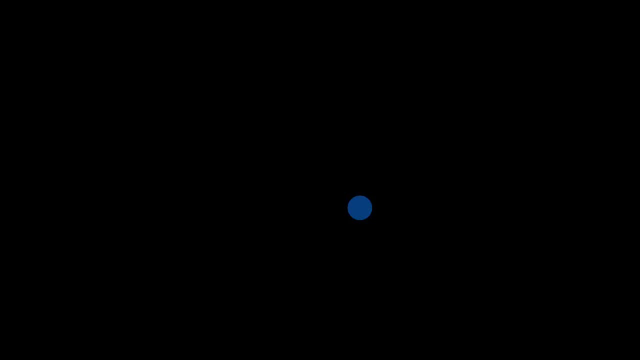 presenting in PowerPoint. There are quite a few different shortcut keys here. You could take a look through these and see which ones will be the most valuable to you. For instance, a few of the things I could do. if I press B, it'll change the slide to black. I could press W to change the. 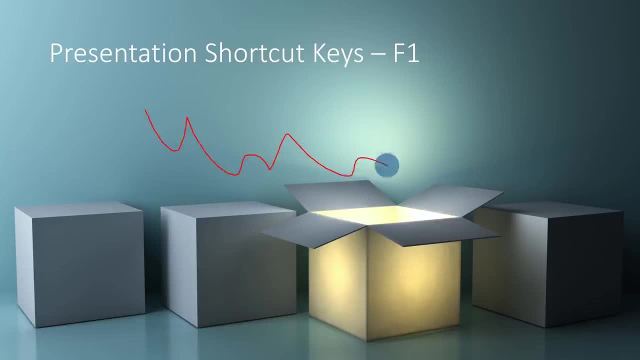 slide to white. I could also press Control P and that'll bring up a pen tool and I can then annotate the screen. I could even bring up a highlighter. I could bring up a laser pointer. There are all these different tools that I have while I'm presenting. 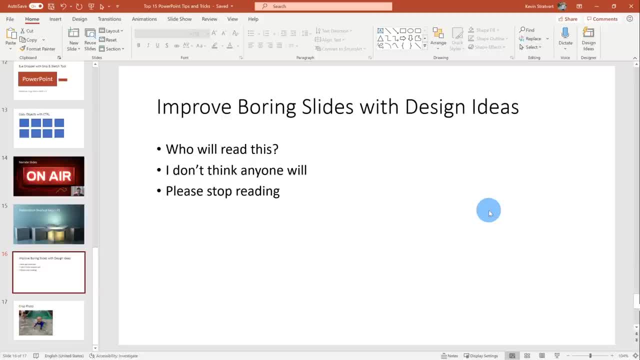 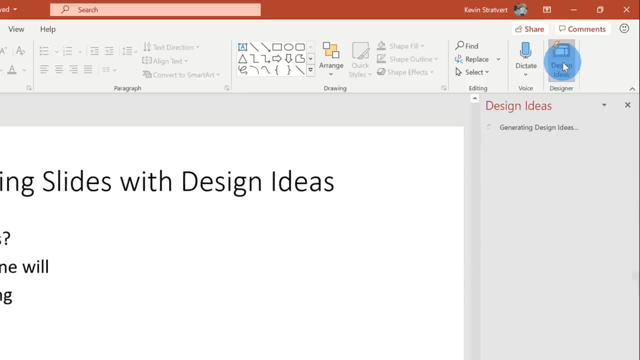 Tip number 14, I want to show you how you could take a boring slide like this and make it a lot more exciting by using design ideas. To use design ideas, click on home on the top ribbon and then over on the far right-hand side. you see an option for designer or design ideas. 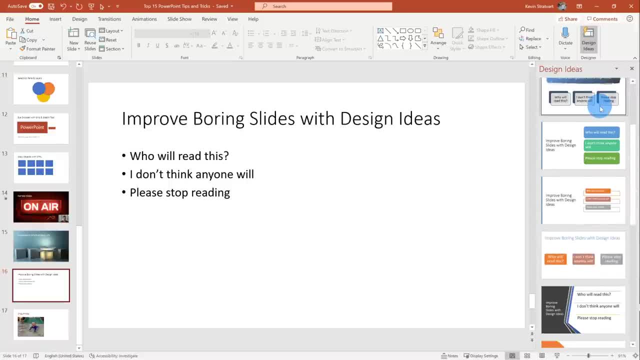 Let's click on this. This now shows me a whole bunch of design ideas on the right-hand side. These are constantly evolving and they're constantly getting better. Now I'm going to click on this first one and let's see how this works. Here it formats my slide in a much more. 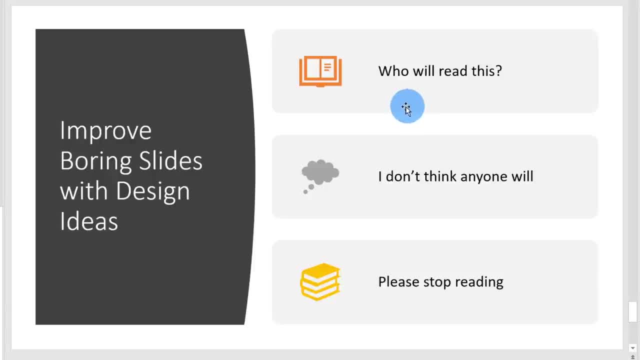 aesthetically pleasing way. Now one of the things that's really neat too, and I don't know if you noticed this, but here the text says who will read this, and here you see a picture of a book. I don't think anyone will. The word think is in there and I see a little cloud. that typically goes along.